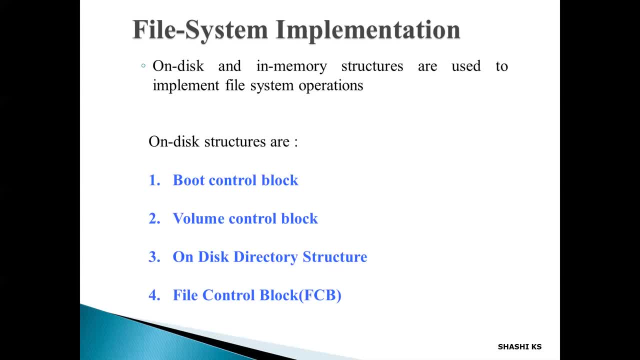 Volume is nothing, but we have learnt while learning about file systems. the volume is nothing but different parts or partitions of a file system may be combined together, the form of a blank volume, Multiple parts of a file system which are not currently holding any file system. 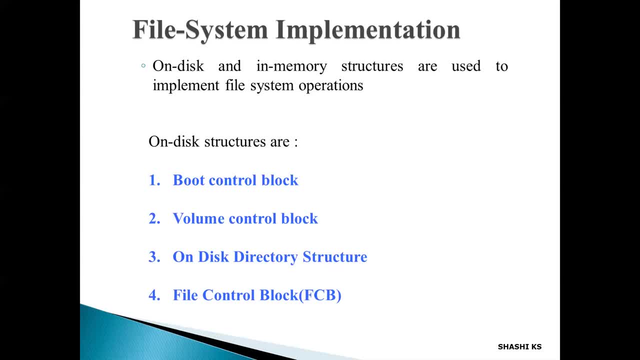 may be combined together to form a volume. So here, for every such volume, a boot control block will be maintained. And what is this boot control block going to store? It is going to store information needed by the computer system to boot an operating system from the 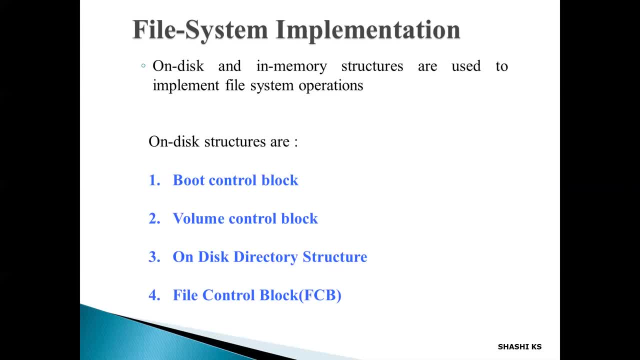 disk. If you are booting an operating system from the disk, then all that information needed during system startup time, during the booting time. all that information is stored in the boot control block. In case, if your disk is not storing any operating system, this boot. 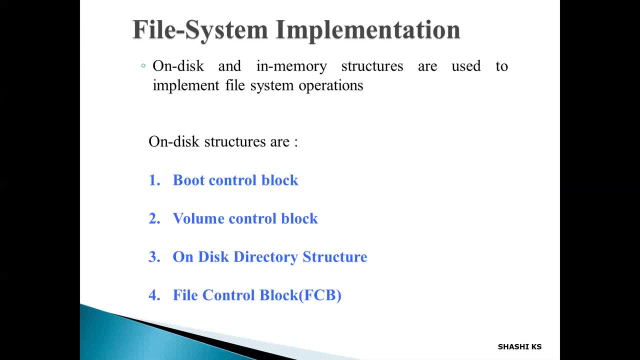 control block will be empty And this will be the first block in any volume, So this will be called by different names. In Unix, boot control block is called as boot block. In Windows NTFS file system this is called as partition boot sector, The next on disk. 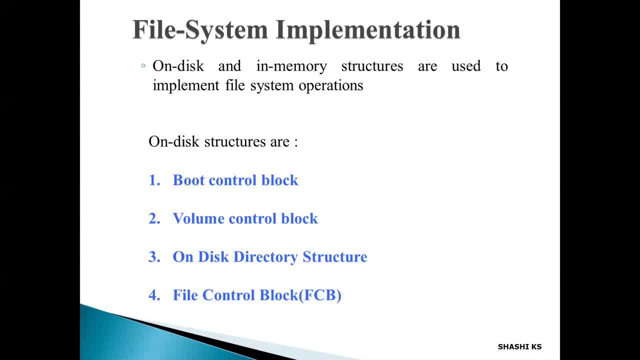 structure is the volume control block. Just now I told you what is a volume. Volume is nothing, but multiple parts, partitions of a file system may be combined together to form volume. So volume is nothing, but you can consider it as a chunk of storage which may be used to hold a file system. So this 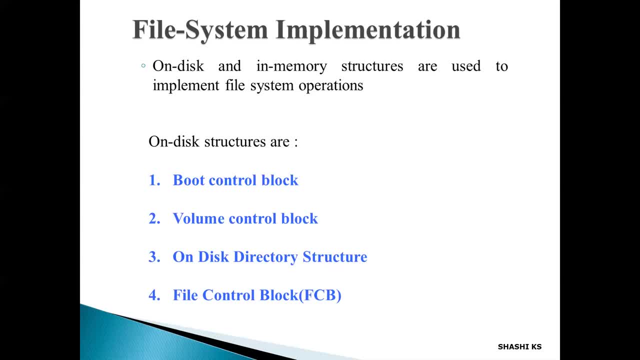 volume control block contains the information about the volume. It contains information about the volume. That is what information it is going to. it is made up of multiple partitions, right? Multiple partitions are combined to form volume, So this volume is a volume control block. It contains information like how many blocks are there in the partition. 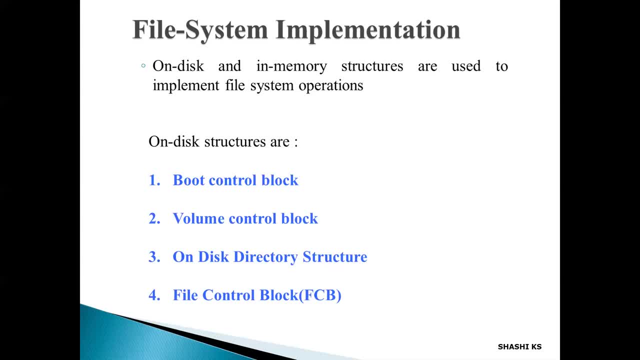 what is the size of the block, what is the free block count and how many free block pointers are there? how many free FCBs are there? FCB is nothing but file control block. So how many free FCBs are there? how many free FCB pointers are there? all that information is. 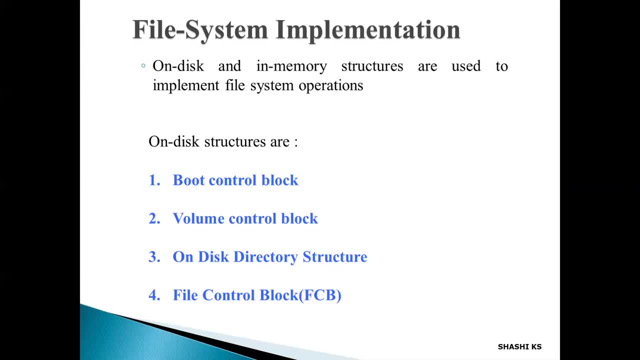 maintained in the volume control block, And this is also called as super block in Unix, And it is stored in the volume control block is stored in the master file table in your Windows NTFS file system. The third one is your on-disk directory structure. Now here: 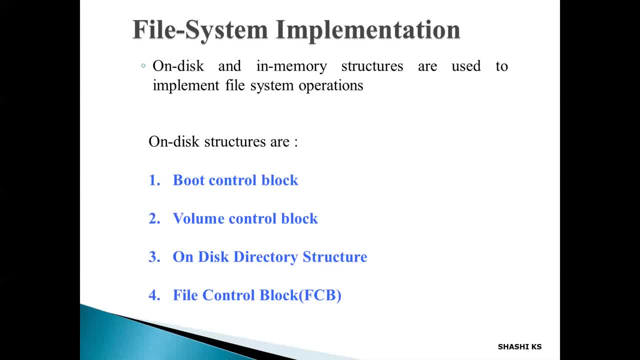 why I am saying on-disk directory structure is we have one directory structure on the memory also. that is called in-memory directory structure. So that is why we call it as on-disk directory structure. Now, this on-disk directory structure maintains frequently accessed file. 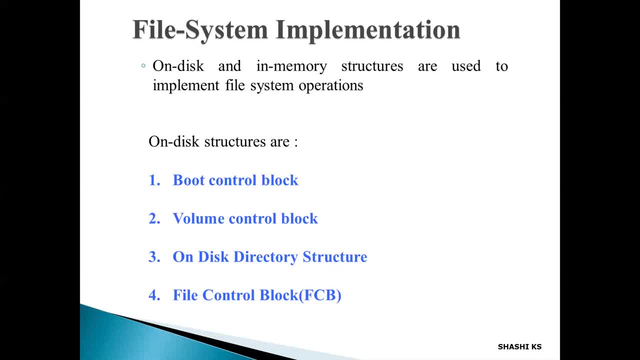 information. All recently accessed file information will be maintained here. So this directory structure contains information needed to organize the files. One directory structure will be maintained for every file system and it contains information needed to organize the files. So the next one is file control block. Sorry, I made a mistake here. On-disk directory structure. 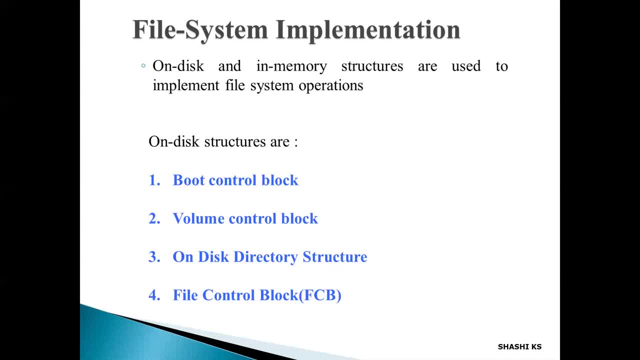 contains information needed to store the file system. In-memory directory structure only contains the information needed to store the file system. So on-disk directory structure contains the recently accessed file information. So ONDISC means it contains information about all the files in the file system. 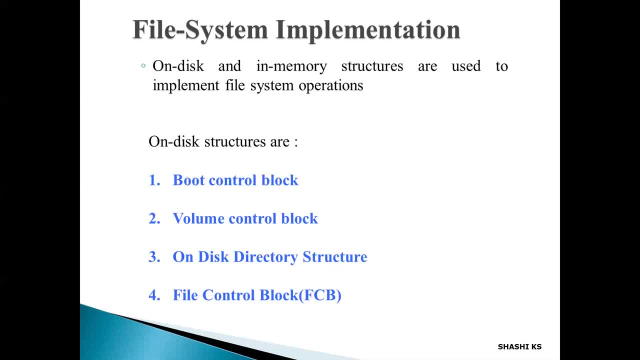 So not only the recently used information. So fourth one is file control block. So file control block maintains information about the file. So what information it is going to store? information about the file permissions, who is the owner of the file, what is the size of? 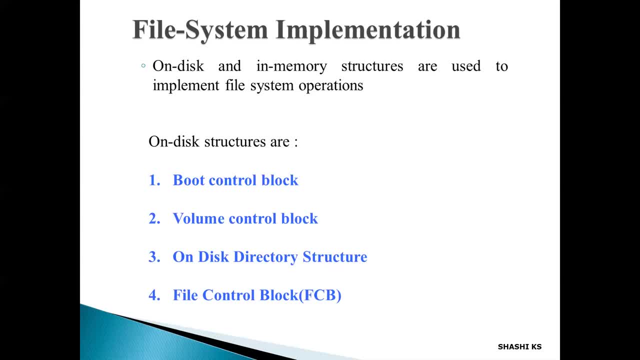 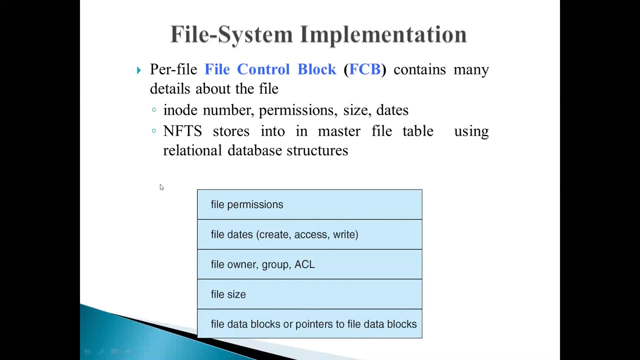 the data blocks of the file. what is the location of the data blocks of the file? all such information will be stored in the file control block. so file control block is maintained for every file. okay, file control block is maintained for every file. so here it shows a sample file control block. in the screen you can see a sample file control block. 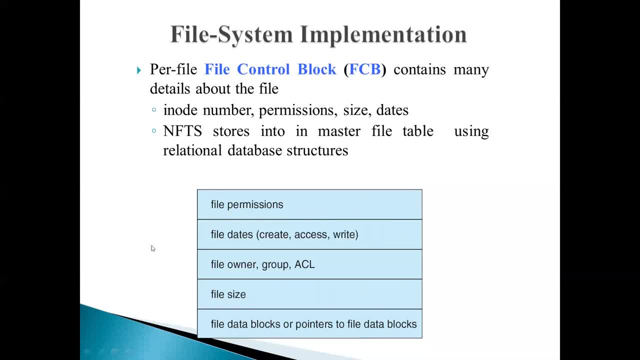 you can see that it stores some information like file permissions, when the file was created, written, etc. file owner, etc. and in unix file system this file control block is called as inode. that's why we have inode number here, and then in ntfs this information about file control block will be. 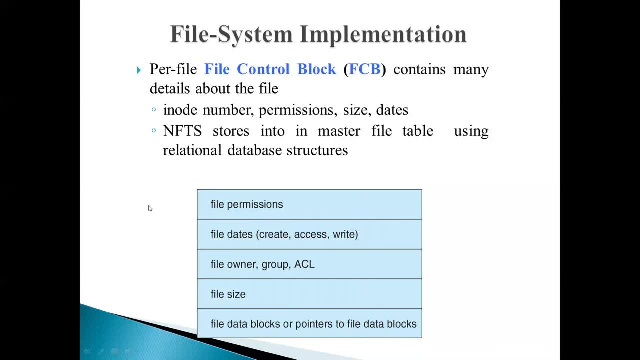 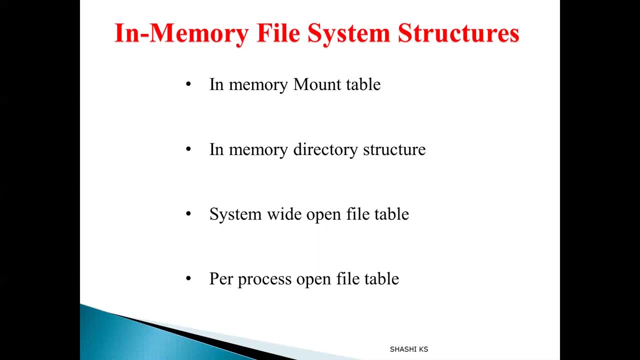 stored in the master file table itself. so that is about the on disk file system structures. what are the on disk file system structures? boot control block, volume control block and then your directory structure on disk directory structure and then your file control block. next is your in-memory file system structures. so you have this is nothing but the. 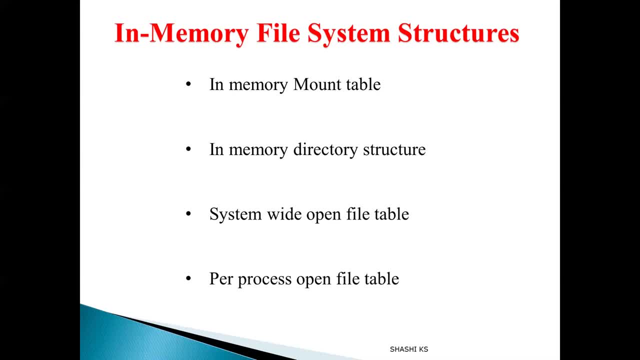 data structures which reside in the memory that is responsible for managing the file system or for implementing the file system. there are four data structures needed for the implementation of the file system. one is in-memory mount table. second one is in-memory directory structure. third one is system wide open file system. 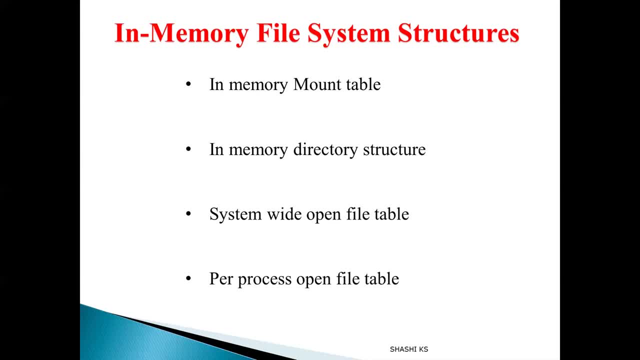 file table. and fourth one is per process, open file table. okay, so first one is in memory mount table. what is the meaning of in memory mount table? so previously i have told you about file system mounting. what is the meaning of mounting? mounting is nothing but attaching a new file system to an 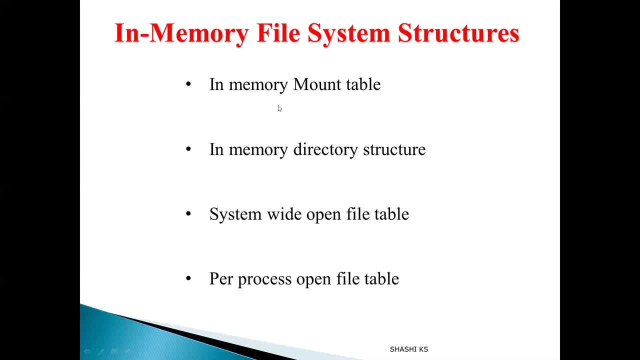 already existing file system. that is called mounting right, and the directory to which you are going to attach your new file system is called as mount point. now this mount table contains information about each mounted volume: which volume is being mounted currently and where it is mounted. what is the mount point. all that information is maintained in the in memory. 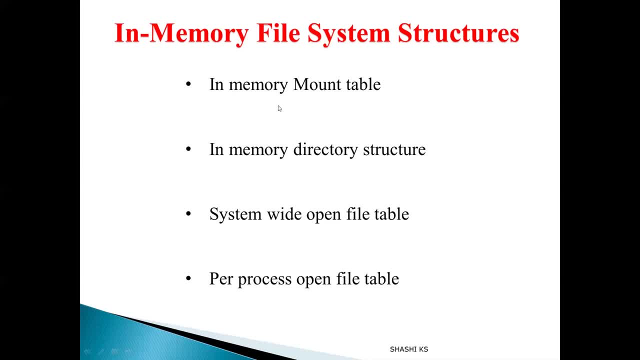 mount table. second is the in memory directory structure. as i told you just now, in memory directory structure stores the directory information of recently accessed files. stores the directory information of recently accessed files and directives. the third data structure is system wide open file table. so system wide open file table. it maintains information about all the files opened by all. 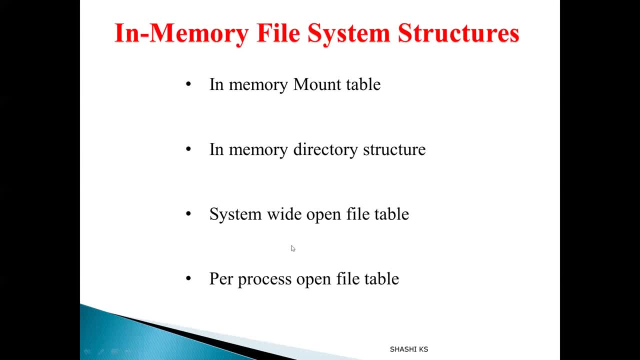 the processes in the system. okay, suppose if you have five processes in memory, what are all the files opened by all these processes? all files which are open in the system currently. every, every such file information will be there in the system wide open file table. fourth, data structure. 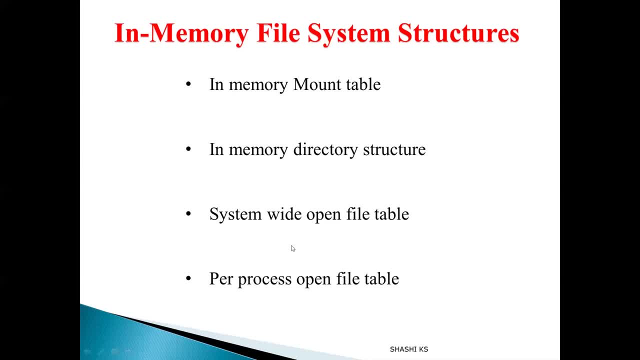 now this part, process open file table contains list of all the files opened by a particular process. okay, if i have process P1, how many files are opened by a process? all that information per process. so so every for every process a separate table will be maintained for P1. P1 has open fire three files. 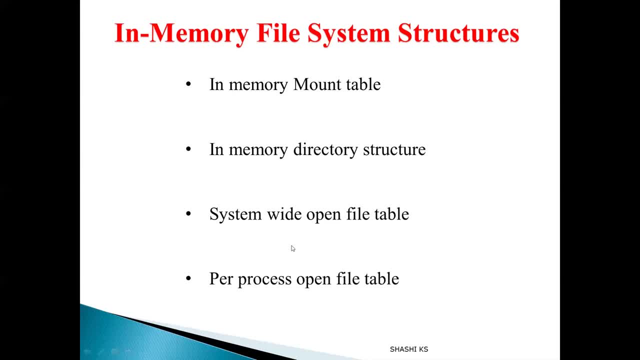 then all those three file information will be maintained in the process open file table and this third process open file table will contain a pointer to the system wide open fire table. now, if i decide to open table, why? because let's say, if two processes have opened the same file, then two entries will not be. 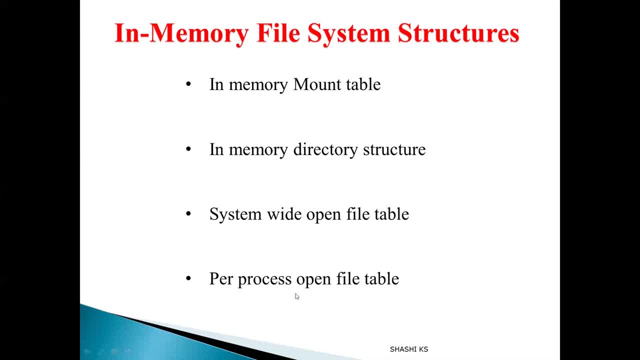 created in the system wide open file table, a new entry will be created for each of those two processes. let's say p1 and p2 are have opened file f1, then a new entry will be there in p1's file table and a new entry will be there in process p2's open file table. but both will be. 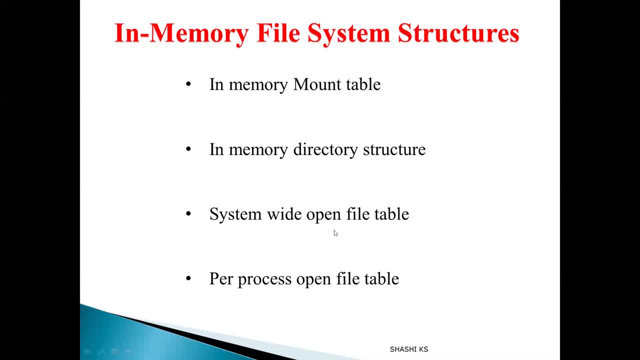 pointing to same entry for the file in the system wide open file table. this is to keep track right, because otherwise it cannot keep track of which process, what are all the processes which which are working with a particular file. so for that no new pointers are maintained, if there will be. 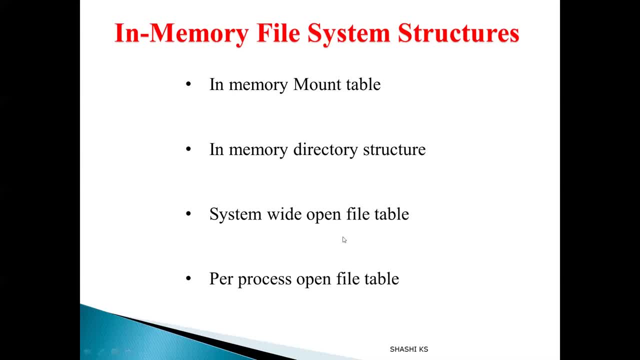 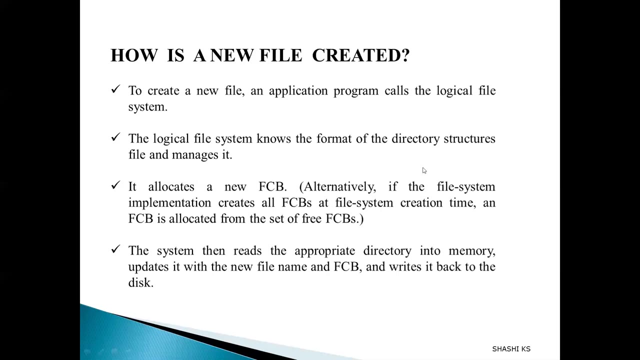 same pointer: both processes will be pointing to the same entry in the system wide open file table for a particular file. so that is about the four types of in-memory file system structures. you so, let's say, a new file has to be created, then what what will happen is to create a new file. 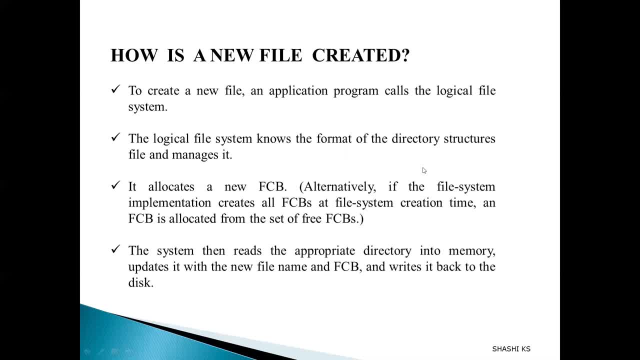 the program will issue the open system, the. it will issue the system called for creation of the file. so then this will in turn call the logical file system. just to recall that, we learned about logical file system by learning about file system structure in the last class, so this logical file system is. 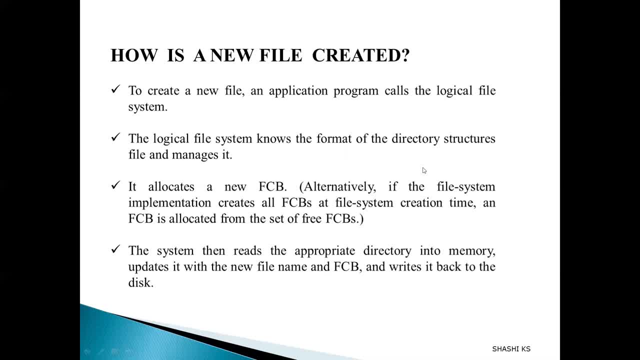 responsible for managing the directory structure. if you can recollect, so it knows the format of all the directories. I alwaysко all data, new CD, any file name and the new series. you provided with. everything return back into the disk or else, if the file is going to be read or written next, 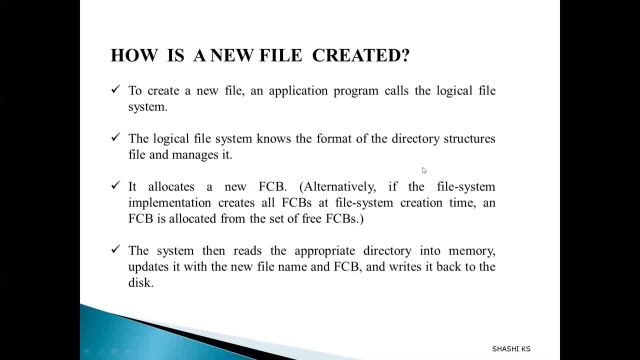 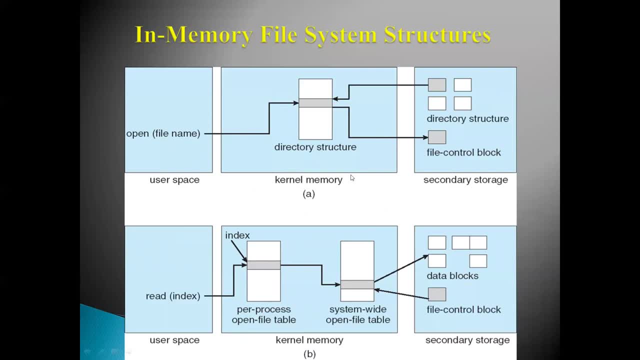 then it will reside in memory. so this is how a new file is created. so next is about how file system operations will be carried out. okay, just try to look at this diagram and listen carefully. so let's say, if a file for a file to be created, it has to be first opened. if a file has been created, we 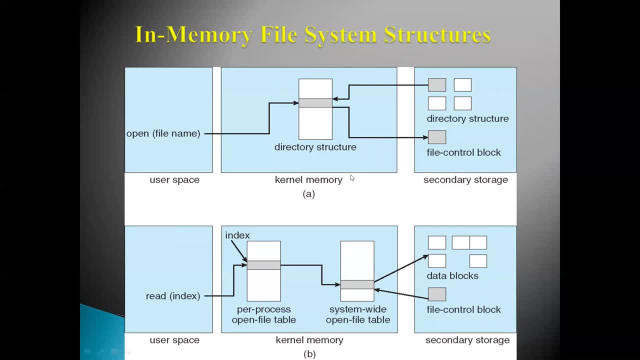 need to work with the file. if the application program has to read from the file or if it has to write from the file, it's straight away. the program cannot read or write from the file. it has to first issue the open system call. so if application program issues a open system call, then what the open system call will? 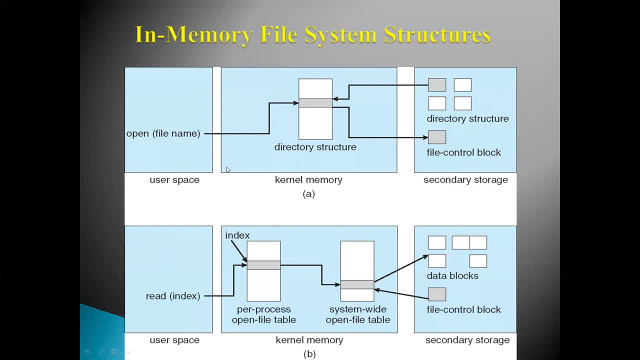 do is open. system call will first check whether an entry for the file is already there in the system-wide open file table. what is the meaning of that? if an entry is already there in the anytime open, it means that the file is already opened by some other process in the system. 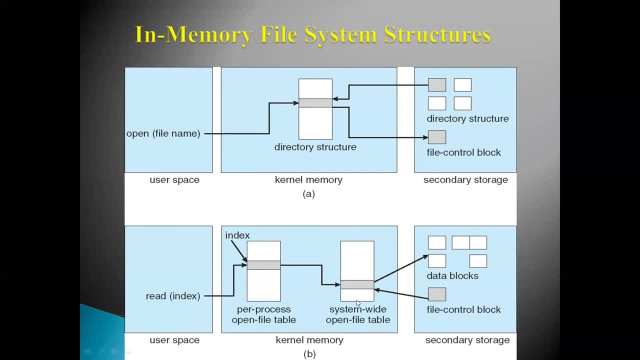 So no new entry should be created because it will create a lot of overhead. So OpenSystemFault will check whether the file is already opened in the system-wide OpenFile table. If it is already opened, then a new entry will be created in the per-process OpenFile table. 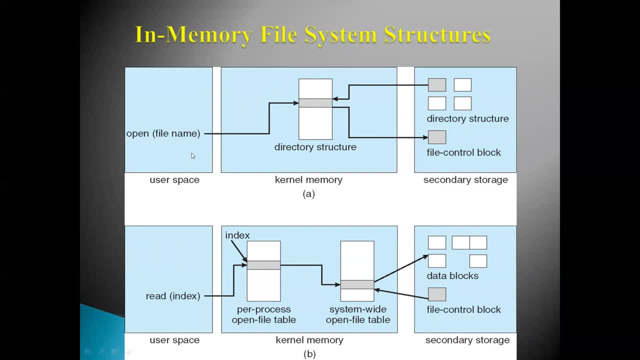 for that particular program which is requesting it, And then that entry will be pointing to the same location in the system-wide OpenFile table because file is already opened. So a new per-process OpenFile table will be created for the currently requesting process and then that entry will be pointing to the entry in the system-wide OpenFile table for that file. 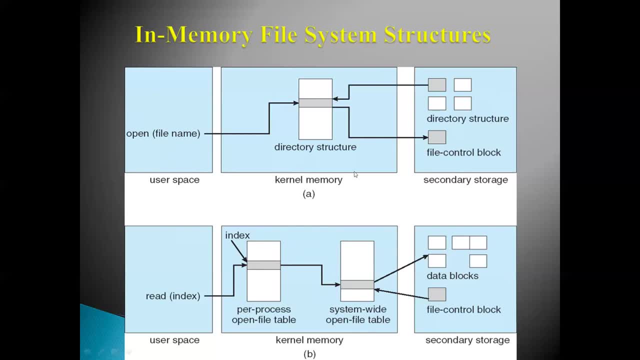 In case if the file is not already opened? now only one program is trying to open a file and it is not already opened, and so its entry is not there in the system-wide OpenFile table. So then what will happen? The OpenSystem call will search for the file control block of this file in the disk. 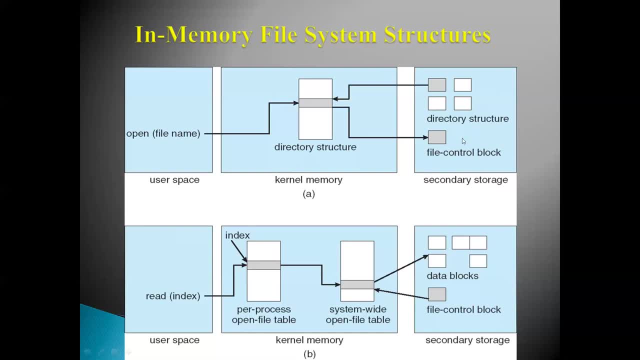 File control block will be there on the disk. It will search the file control block Already. I told you file control block contains the information about the file. So to work with the file this file control block has to be brought into memory. So it will check whether the FCB is there in the disk. 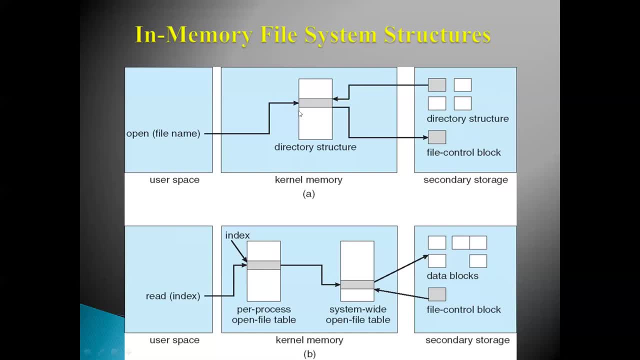 and it will bring that from the disk into the memory. Once that is brought from the disk into the memory, a pointer will be created. The OpenSystem call returns a pointer to the appropriate entry for the file in the per-process: OpenFile table. 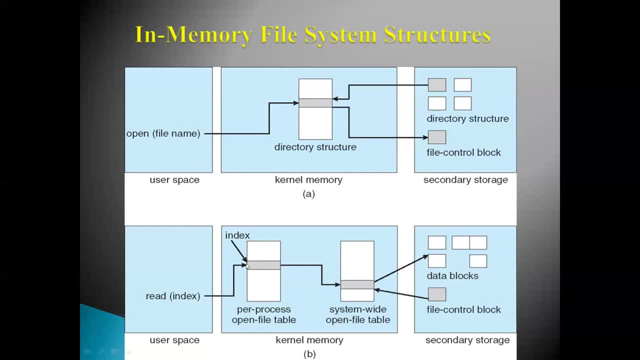 You can see that index is the pointer here. Why do I need this pointer? Because after this I am just now talking about OpenSystem call. After that, if the process wants to do read operation, it can make use of this pointer Through this pointer. 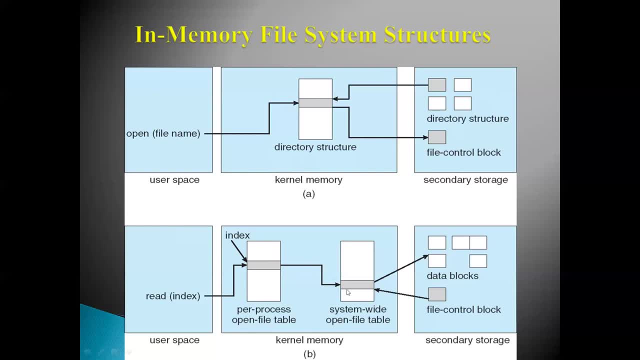 it will know the location of the file on the system-wide OpenFile table. Through that it will know the location of the file control block of the file, So it can work with the file. For that it needs a pointer. The pointer pointing to the appropriate entry for the file in the per-process OpenFile table will be returned. 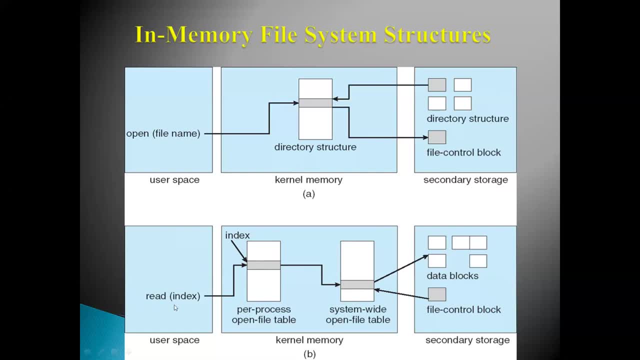 After that- let's say the program wants to do a read operation on the file- it will make use of that pointer to access that particular file's entry in the per-process OpenFile table. After that, the OpenSystem call brings the file control block of the file into memory. 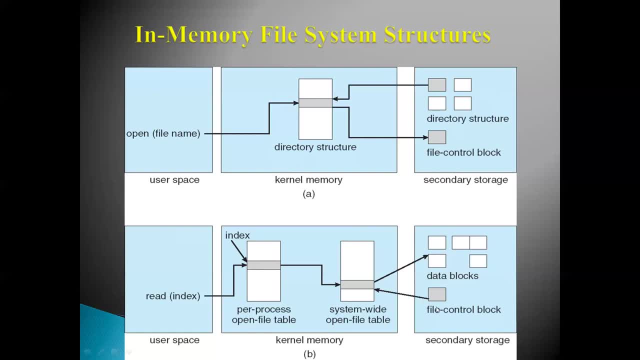 So this diagram or this diagram both represents the same thing. The file control block of the file in the disk is brought into memory And then a pointer will be returned by the OpenSystem call. This pointer will be pointing to the appropriate entry for the file in the per-process OpenFile table. 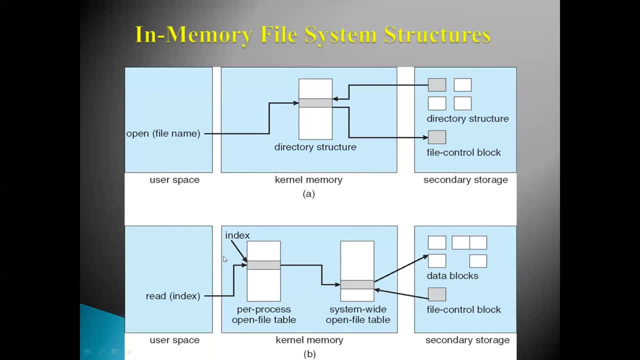 And from there on, this pointer will be used to access that particular file. If a read operation has to be done on the file, this pointer will be used. If a write operation has to be done on the file, this pointer will be used. 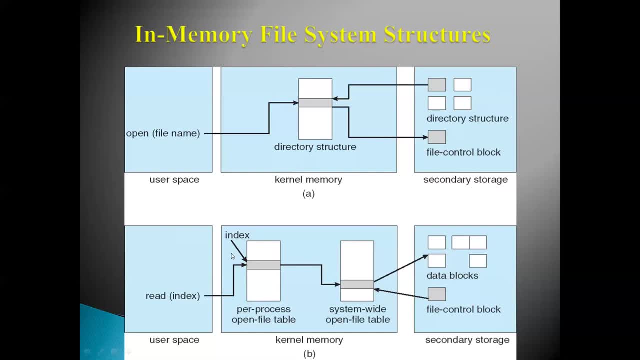 And then when all the file operations are over, then when the closed system call is issued, then the file control block which is residing in the memory will be removed and it will be placed back into the disk. The per-process table entry for that file also will be removed. 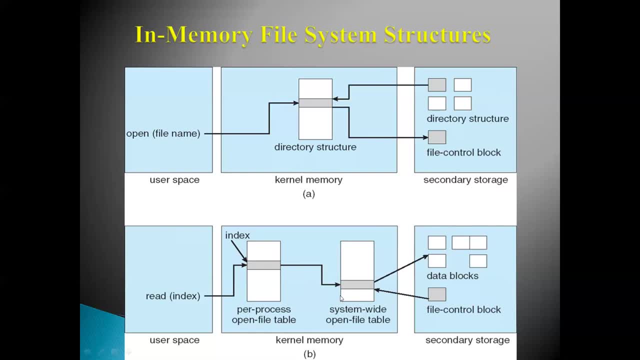 And system-wide OpenFile table count also will be removed. And system-wide OpenFile table count also will be removed. In this way, all the files which are opened will be kept track of by the operating system. In this way, all the files which are opened will be kept track of by the operating system. 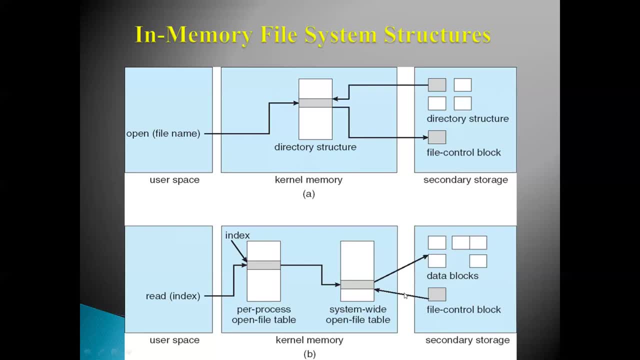 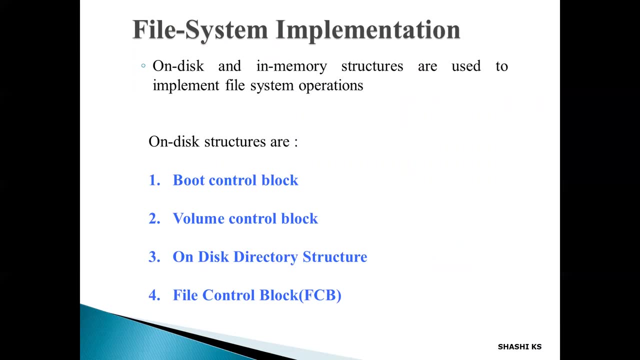 So this is all about file system implementation. So this is all about file system implementation. So I'll just repeat: We just saw that there are four on-disk structures responsible for file needed for file system implementation: Boot control block, which contains the booting information for the operating system on the disk. 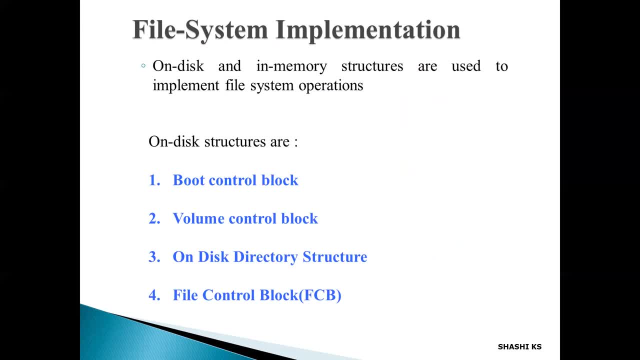 Volume control block maintains information about file. Volume control block maintains information about partitions on the volume. On-disk directory structure maintains the file information. maintains the file system information maintained by the directory. File control block maintains information about the file, like file ownership, permissions, size, etc. 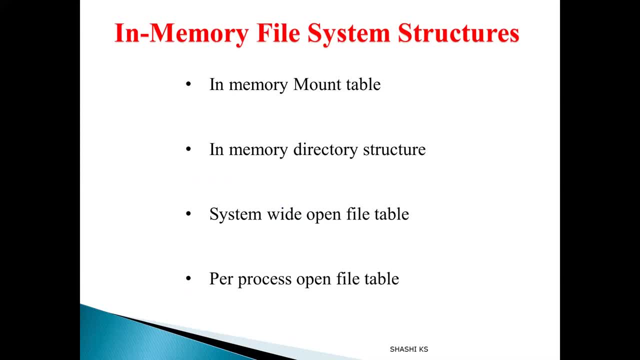 And then we saw about in-memory file system structures, which consists of mount table. Mount table maintains the file system mounting information, Then directory structure- in-memory directory structure maintains the information about recently accessed files and directories, And then we have system-wide open file table. 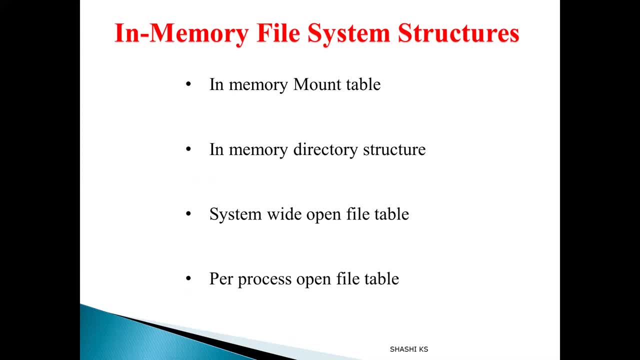 which contains list of all the files opened by all the processes in the system. Then we saw about per-process open file table, which will maintain, for every process, all the files opened by the process. That information will be there in the per-process open file table. 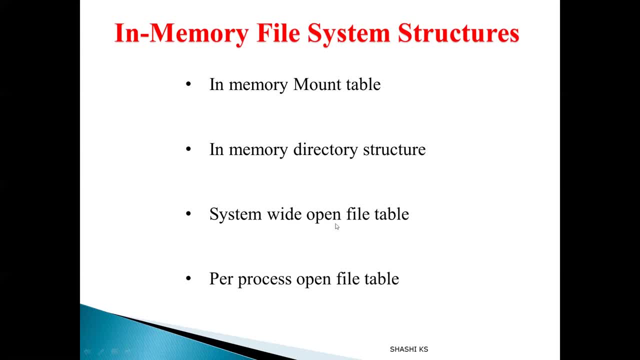 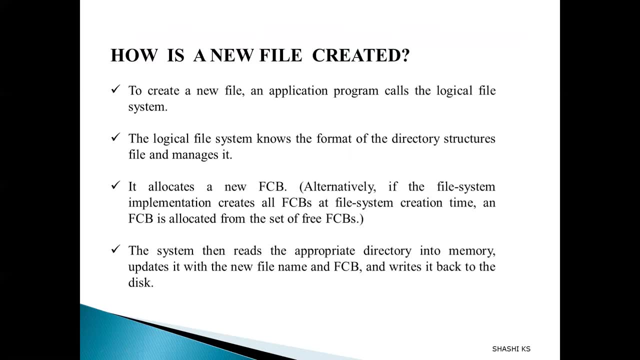 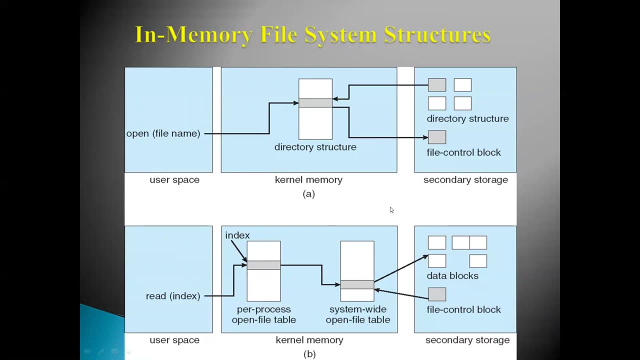 This always will contain a pointer pointing to an entry for that file which it has opened In the system-wide open file table. Then we saw how the file system operations are implemented with the open system call, read system call and when a closed system call is being issued. 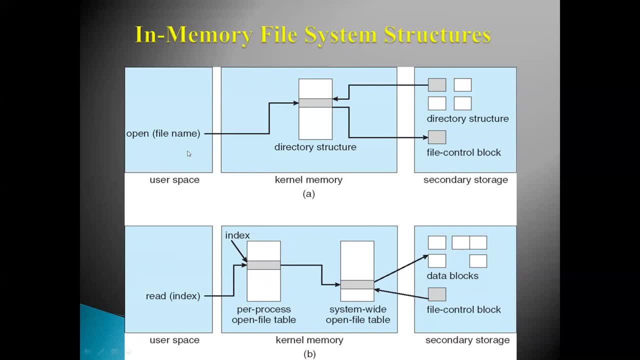 Whenever we try to open a file, the open system call will first check if the file is already opened by checking the system-wide open file table. If it is already opened, it will just create a new entry in the per-process open file table. 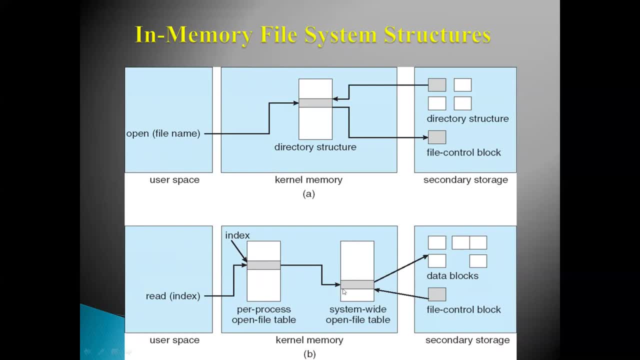 And the new entry will be pointing to the same old entry in the system-wide open file table, And if the file is not already opened, then the file's FCB of the file will be brought from the disk into memory. And then, once the FCB is brought into memory, 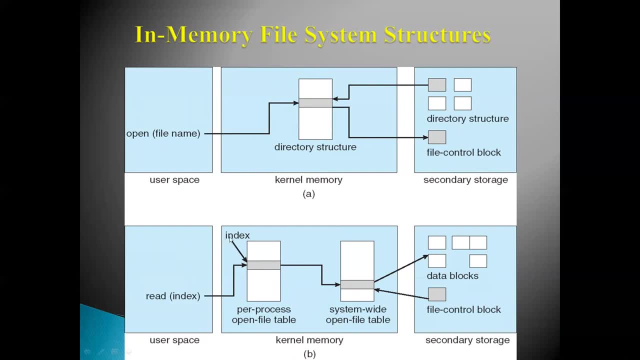 open system call will return a pointer pointing to the appropriate location of the file in the per-process open file table. From there on, all the read-write operations on the file will be done via this pointer And then, when the process has closed, the file. 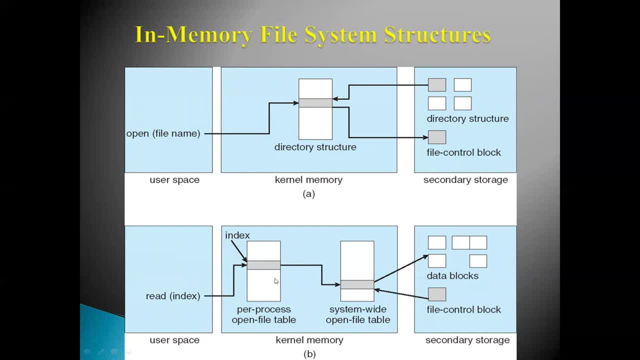 then the entry for the file will be removed from the per-process open file table And the count also will be the open file. count of that particular file will be decremented in the system-wide open file table. Why I am only decrementing, why I am not deleting, is: 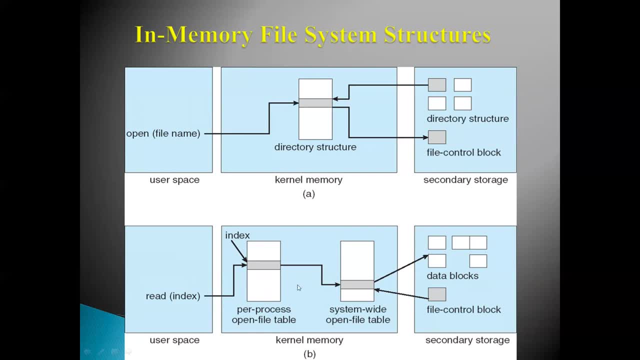 that file is closed by this particular process, It might be opened and still be in working condition by other processes, So only the count will be decremented in the system-wide open file table. So that is all about how file system operations are implemented using the file system structures. 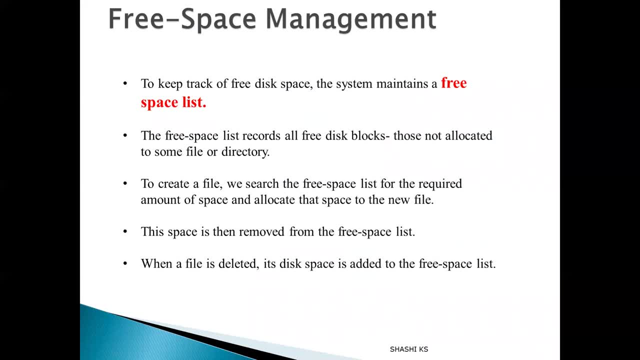 So next topic is about free space management. So what is this free space management? We are having disk space right. We are utilizing the disk space to implement the secondary memory, And this disk space is very limited. So whenever the disk space becomes free, 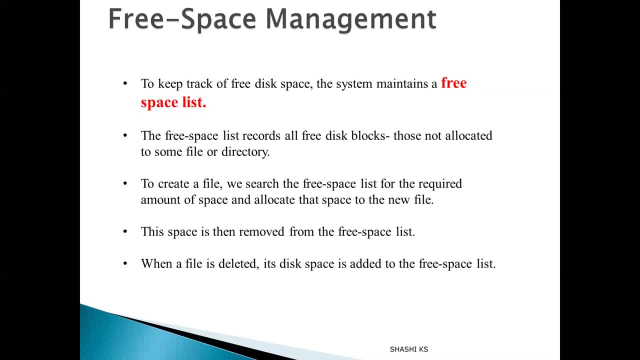 when a file is deleted, disk space becomes free. That free disk space has to be reused. The space which the OS gets by deleting the files on the disk has to be reused. That is called as free space management. Free space management deals with how to reuse the space. 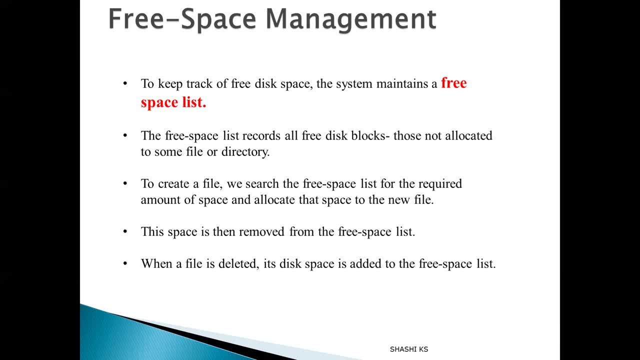 which we get by deleting the files from the disk. How to reuse the space which we get by deleting the files from the disk is called as free space management. For this, the operating system maintains a data structure called as the free space list. Now this free space list will contain a record of all the free disk blocks. 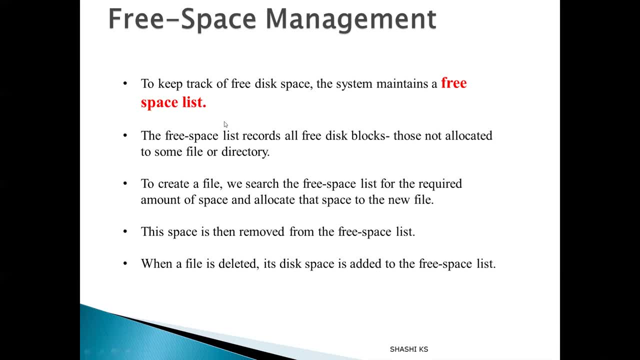 What do I mean by free disk blocks? Blocks which are not allocated for storing any file information or any directory information are called free disk blocks. So whenever a new file has to be created, the OS will check the free space list for space, And whenever a file is deleted, 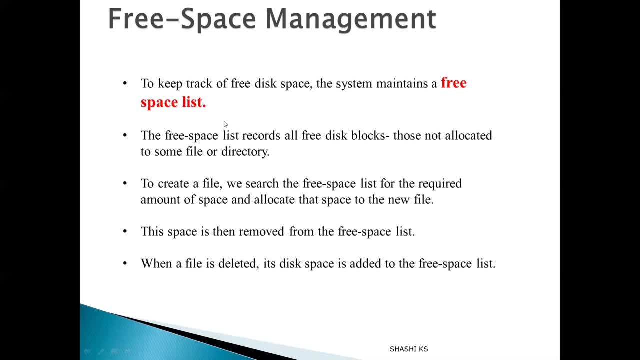 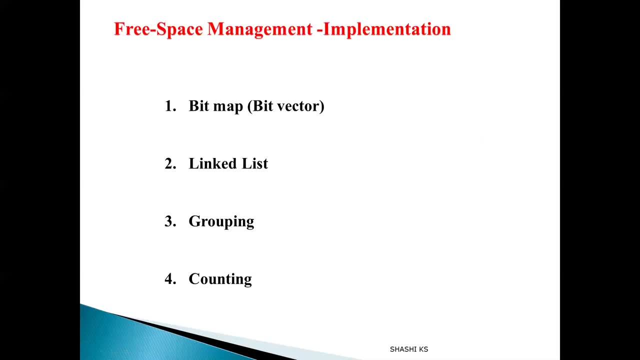 OS will remove that deleted space and add it to the free space list. That is how it is being managed. Now, how can we implement this free space management concept? This implementation of free space management can be done by using four different types of methods. 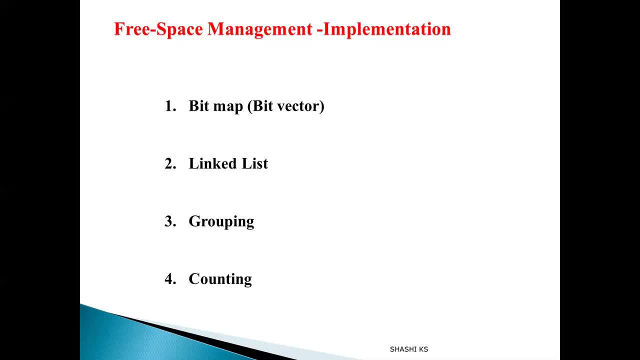 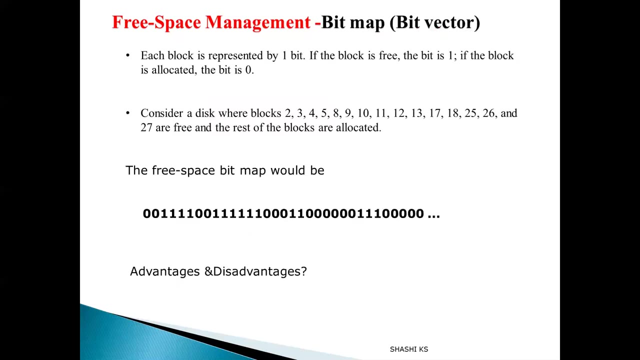 First method is by using bitmap or bitvector. Second method is by using linked list. Third method is by using grouping And fourth method is called as counting. Now let's see about each of these methods in detail. The first method of implementing free space management. 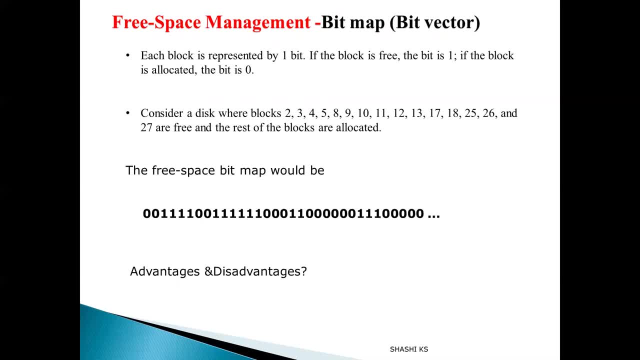 is by using bitmap or bitvector. It is very simple and easy to implement. So what is this bitmap or bitvector? Each block will be represented by one bit. Okay, Which resides on the disk Will be represented by one bit. If the block is free, the bit will be set to one. 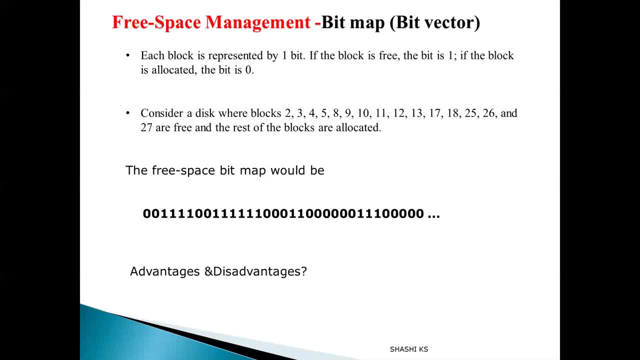 If the block is allocated, the bit will be set to zero. Okay, So free means one, Allocated means zero. So let's say you have a particular disk set of blocks where- and remember that the bitvector will start with block number zero- 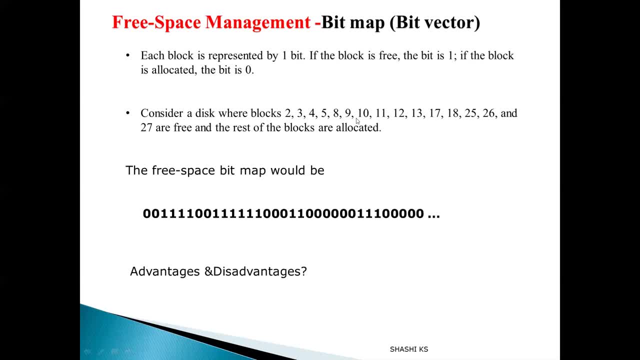 And so here let's say your block numbers: two, three, four, five, These are all the free disk blocks. numbers Okay, Two, three, four, five is free. Eight, nine, ten, eleven, twelve, thirteen is free. 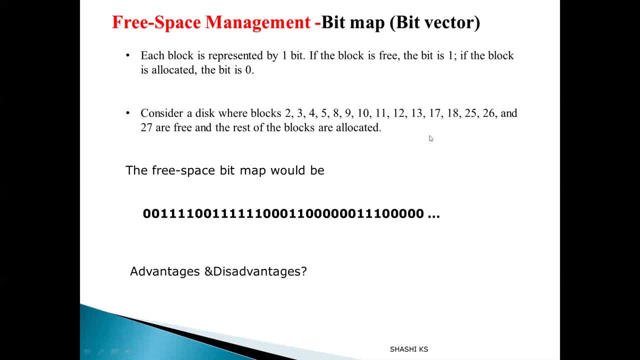 Seventeen, eighteen is free, Twenty-five, twenty-six, twenty-seven is free, And so on. Let's say, if you have a disk like this, where these block numbers are free, Then how will our bitmap or bitvector will look like this: 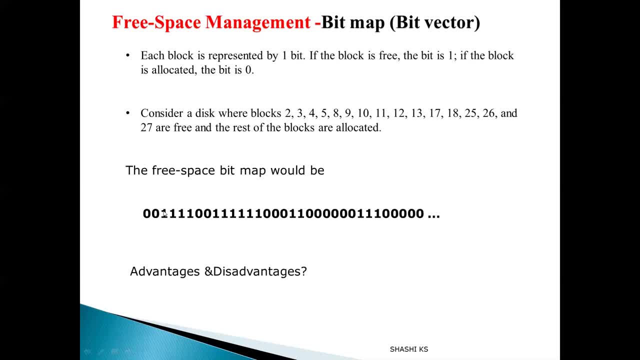 See, this is for zero, This is for one, This is for two. Okay, Two, three, four, five is free. So two, three, four, five, All these bits bitmap is set to one Okay, Indicating that it is free. 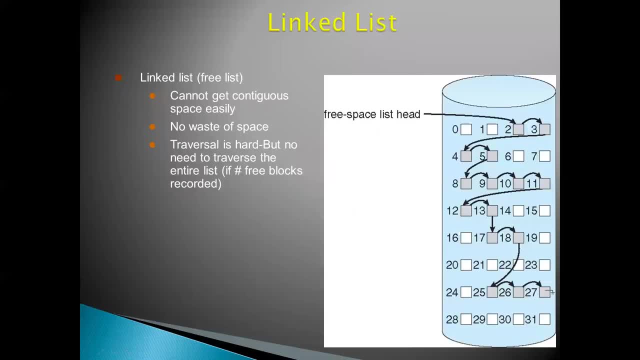 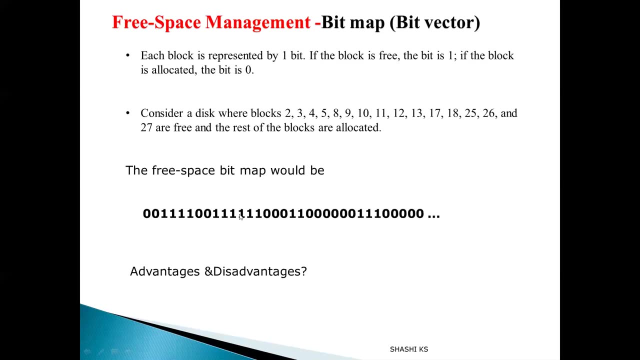 Next is six is free. Next is six. seven is set to zero, Indicating that it is occupied. Then eight, nine, ten, eleven, twelve, thirteen. All this is set to one because they are free. So if it is set to one, it means it is free. 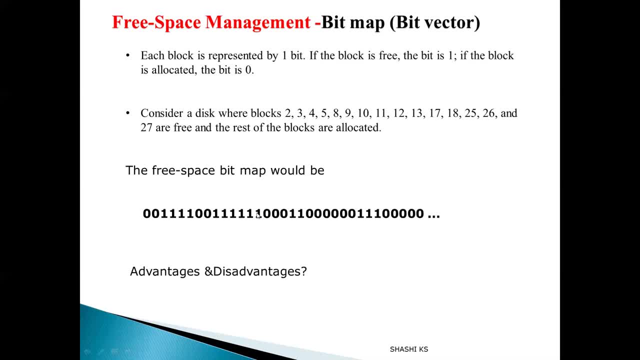 And if it is set to zero, it is occupied. So this is how we use the bitmap, or bitvector, to indicate, to identify the free disk blocks on the disk. So what is the advantage of this approach? As I told you, it is very simple and easy to implement. 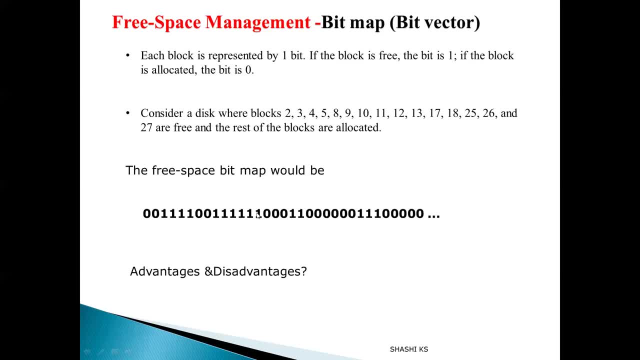 And it is efficient also because you can find the first free disk block very easily Just by looking at the bitmap. we know that if the bit is one, that block is free. Or if you want to find n consecutive free blocks on the disk, that is also very easy. 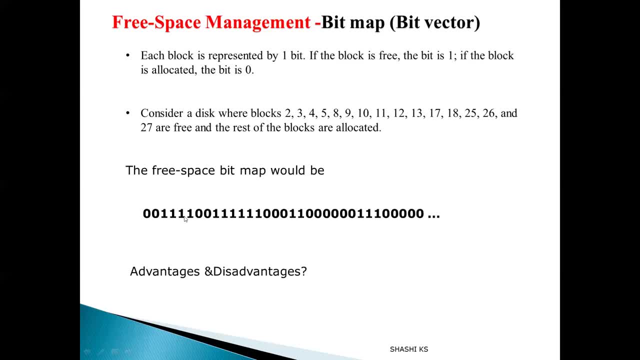 You can see here that consecutively all are one. This means all these are consecutive free disk blocks. So finding the first free disk block is easy. Finding n consecutive free disk blocks is also easy, And many operating systems provide bit manipulation instructions. 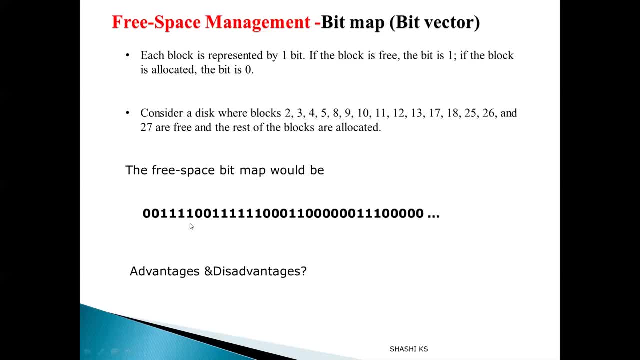 So with that we can easily implement this bitmap concept. So this is the advantage of this concept. But the disadvantage is, if you want this scheme to be efficient, you have to keep the entire bitvector in the memory, Otherwise you cannot find which block is free, which block is occupied. 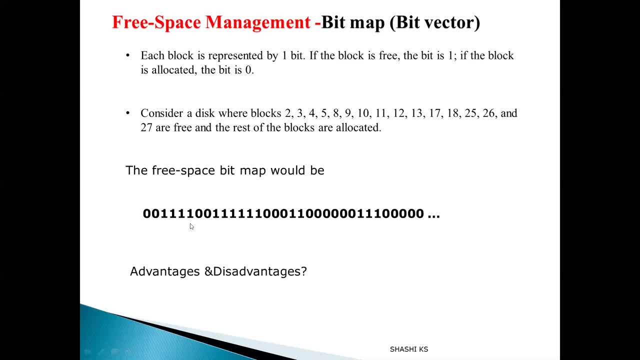 But that is not feasible in all the situations. So if your hard disk size is big, you are going to store more number of disk blocks on the disk. So let's say you have a 40 GB hard disk And each of your block size is 1 KB. 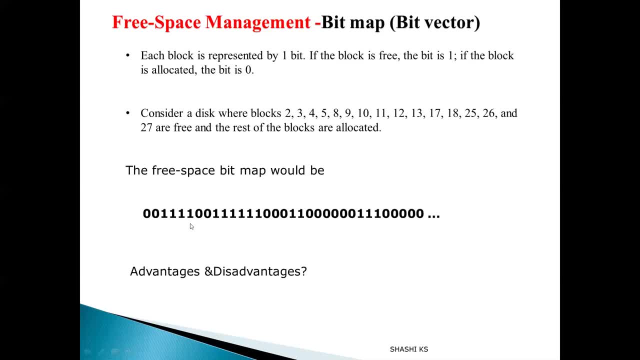 Then in that case your bitmap vector size will be around 5 MB. So then, storing bitvectors of all the disk blocks, of all the file systems, is going to be a very tedious task, Or it might be. it's not possible also. 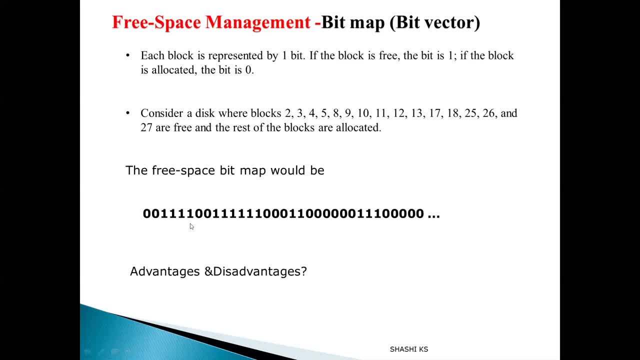 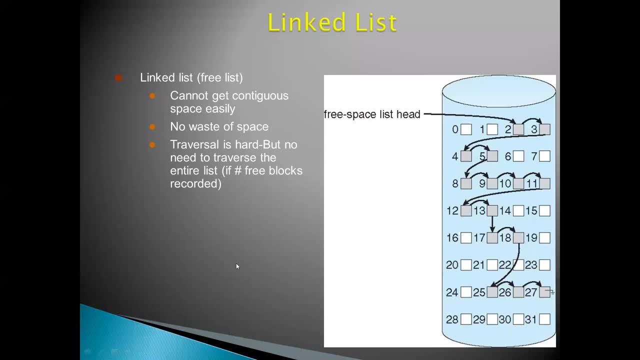 So that is the disadvantage in this bitmap technique. The second method is called as linked list implementation. This is another approach to free space management. There, as the name implies, linked list. What we are doing is all the free disk blocks are linked together by using pointers. 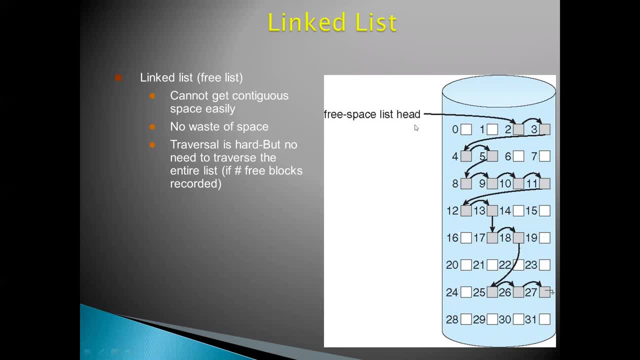 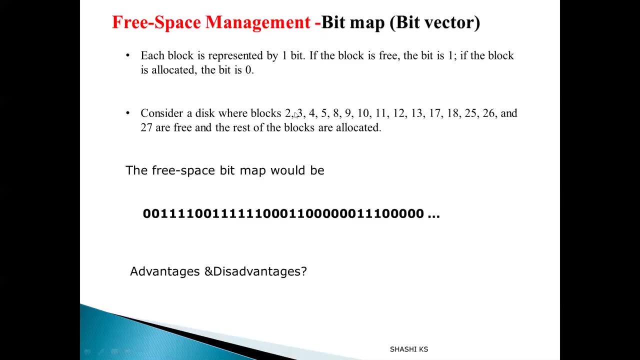 So here you can see in the diagram you have a free space list head. I have used the same example. Just now I told you this: 1,, 2,, 3,, 4, 5 is free. So the first free disk block is 2.. 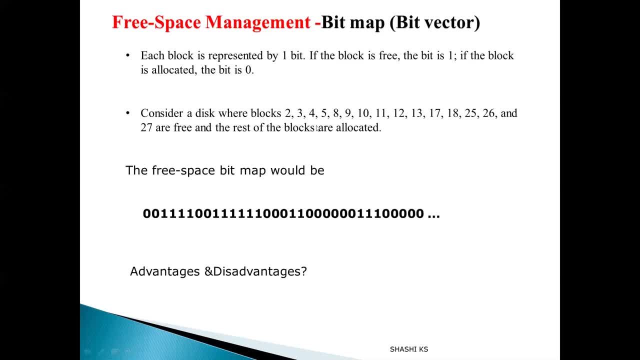 Remember this example, So using the same example for all the next 3 implementations also. So 2,, 3,, 4, 5 is free. 8,, 9,, 10, 11 is free. 8,, 9,, 10,, 11,, 12,, 13 is free. 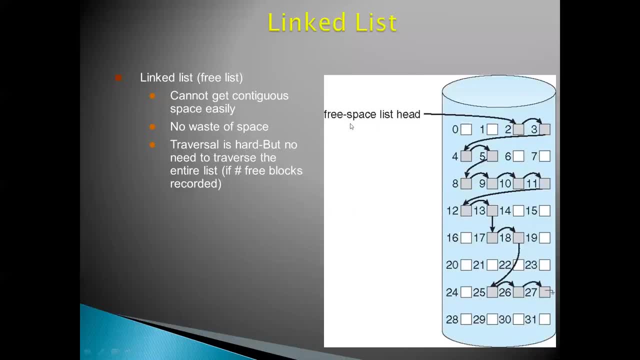 So free space list head will point to the address of the first free disk block. First free disk block is 2.. So this 2 will contain the address of the next free disk block. Then 3 will contain the address of the next free disk block. 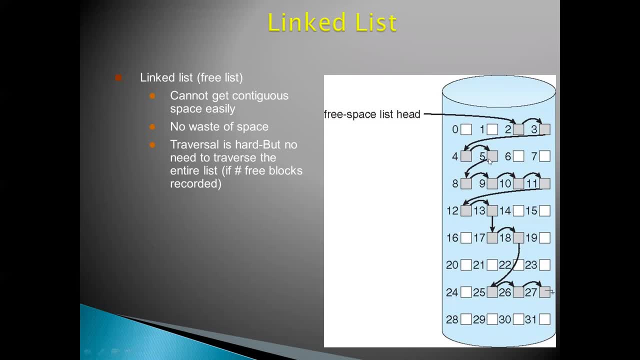 4 will contain the address of the next free disk block, which is 5.. 5 will contain the address of the next free disk block. 5 will contain the address of the next free disk block, disk block, which is 8, and so on. so this is how linked list implementation is done. so it so here. 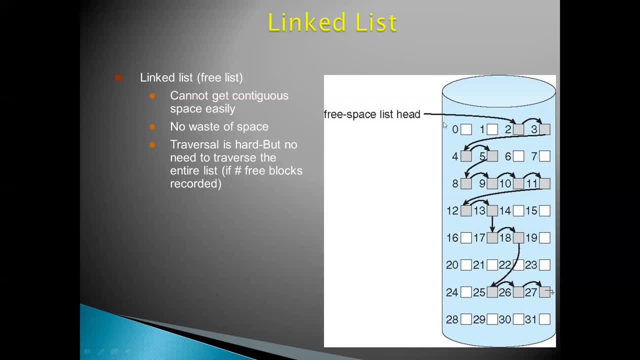 the free space header- free space list header- will point to the first free disk block. that first free disk block will contain a pointer pointing to the address of the next free disk block, and so on. so, with the help of pointers, every block will contain the address of the next free disk block. 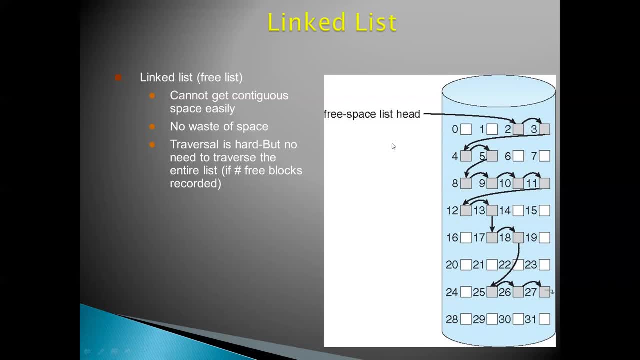 on the disk. so this is how we maintain the linked list implementation. okay, so what is the? uh? what is the disadvantage in this method is we cannot get contiguous space easily, right? so if you want to know the details of contiguous disk space, we need to traverse the 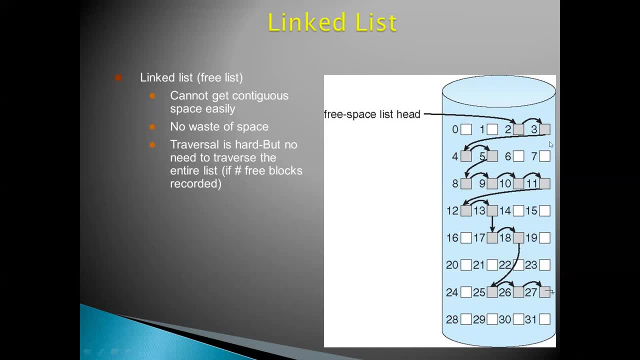 entire uh free space list, because each disk block contains the address of the next free disk block. so i have to traverse through two and then three, and then four and then five, and then i will know the address of the next disk block. all right, so now, if we are keep on moving up ahead, we have 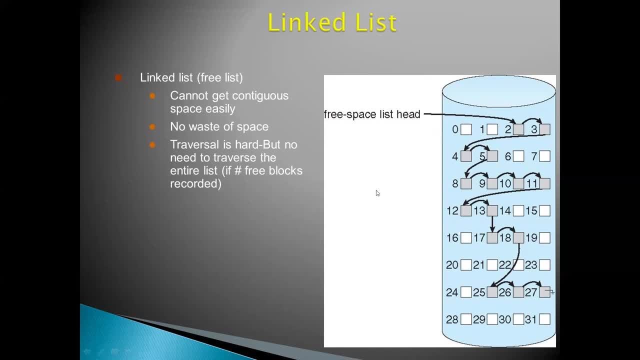 that 6 is not contiguous. So to get contiguous disk space I have to start from the first free disk block and traverse through all the pointers to get a list of all the contiguous disk space. And traversing the list is not efficient because we have to read each block. 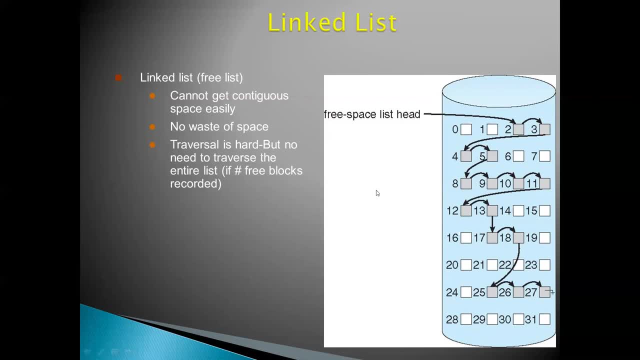 to find the address of the next free disk block. So that is going to take good amount of input output time. So that is the disadvantage here. Traversing the linked list is hard because we have to traverse each and every free disk block to get the address of the next free. 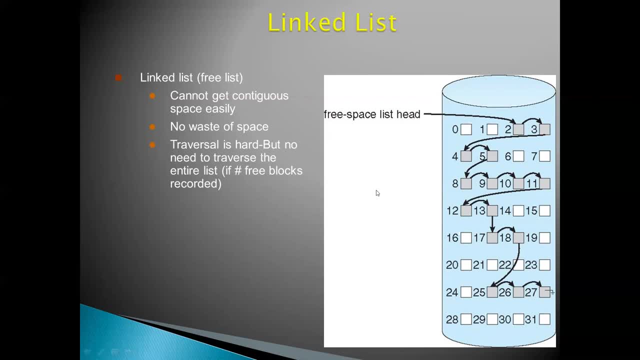 block And so we cannot get the contiguous space easily. But then the advantage is there is no wastage of space. All the free disk blocks are. we are keeping track of addresses of all the free disk blocks and we will be able to utilize them for the file system. 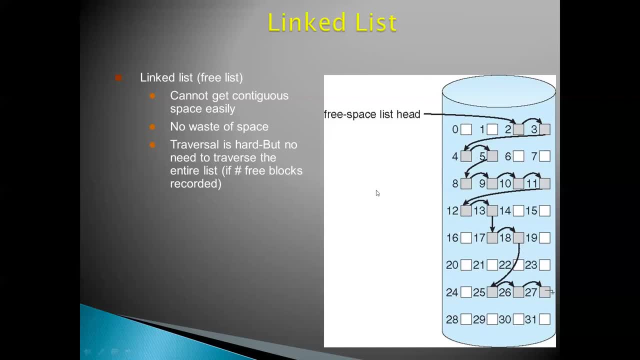 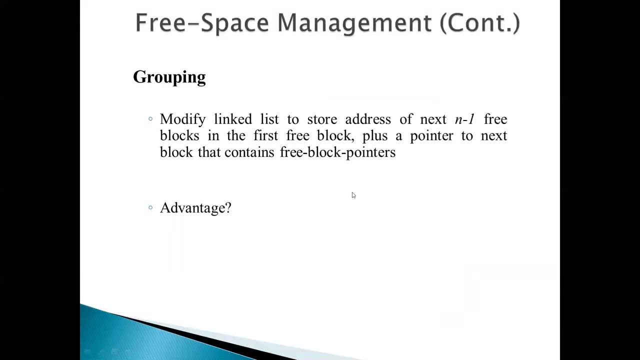 So there is no wastage of space, And so that is about the linked list implementation. And the third type of implementation is called grouping. So here what we do is the linked list implementation is little bit modified. So what we do is let us say: you have n free. 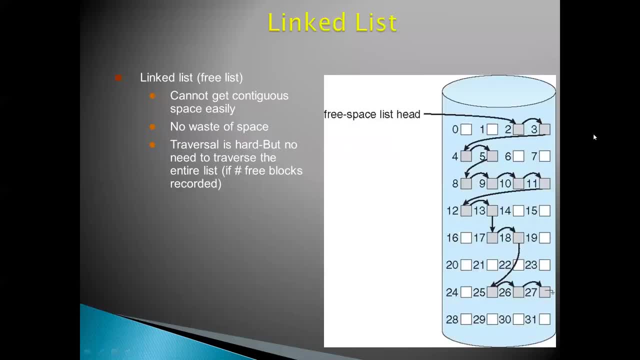 disk blocks: See our same example. we had 2,, 3,, 4, and 5 free. So what 2 will do is it will store the addresses of remaining n-1 free disk blocks. So 2 is not free, So I am. 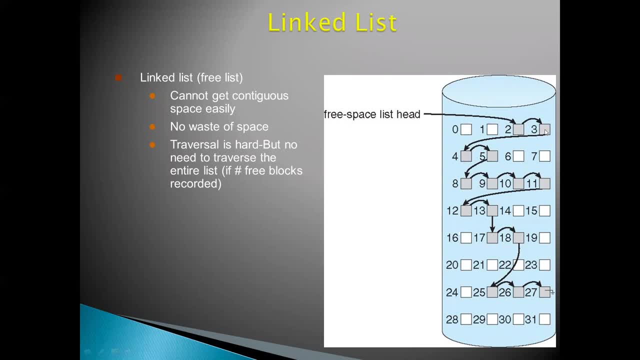 not sure how much is the number sub of jávegas free. it is going to store the addresses of 3,, 4 and 5.. But 3,, 4 and 5 are actually free. that can be used for any particular file. So free space header will point to the first. 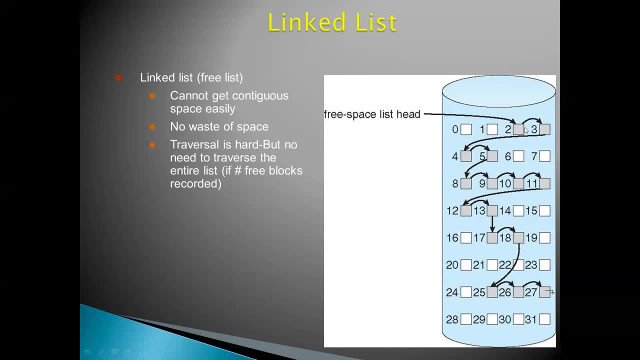 free disk block. The first free disk block will contain n-1 addresses. will contain the addresses of remaining n-1 free disk blocks. So that means 2 will contain the addresses of 3,, 4 and 5 which are remaining n-1 free disk blocks. 8 will contain the addresses 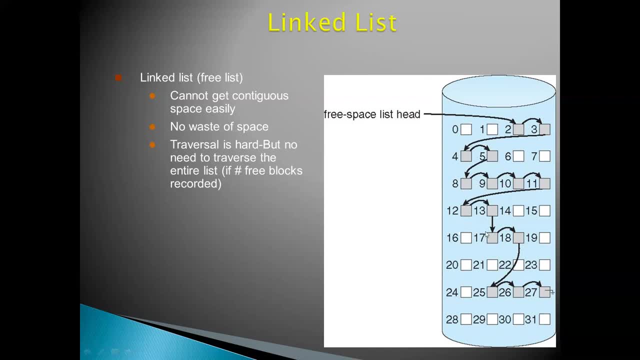 of 9,, 10,, 11,, 12 and 13.. 17 will contain the address of 18 and so on. So the first block in any contiguous in any, the first free disk block, will contain the addresses of next. 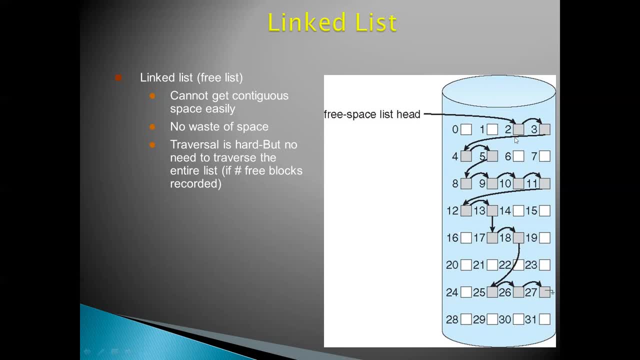 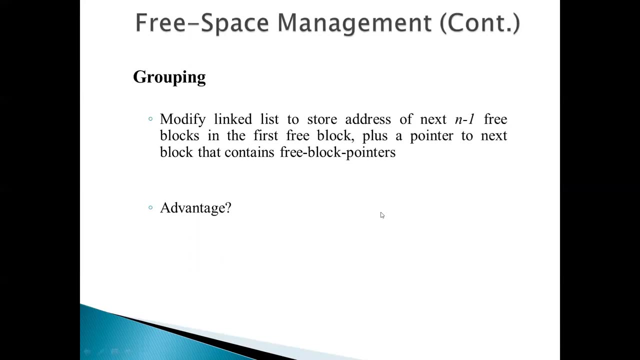 n-1 free disk blocks. So that scheme is called as grouping. Grouping is nothing, but you take the first free block, store the addresses of next n-1 free blocks in the first free block, And the last block will contain the addresses of next n-1 free disk blocks. So 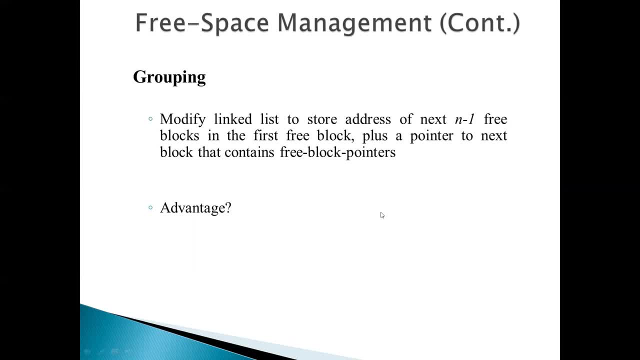 we have seen the grouping scheme where the first free block was contained and then the last free block was containing the addresses of another n-1 free blocks and so on. So the advantage of this grouping scheme is, if you want to find the addresses of large number, 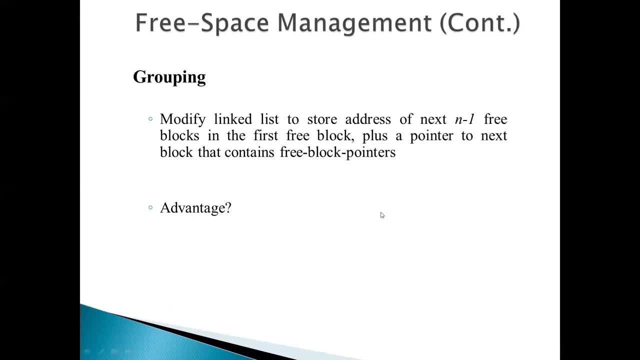 of free blocks in the link list scheme you have to traverse and getting contiguous space was very difficult because you have to traverse each and every disk block to find the addresses of the next free block right and check whether that block is free or not. And check whether 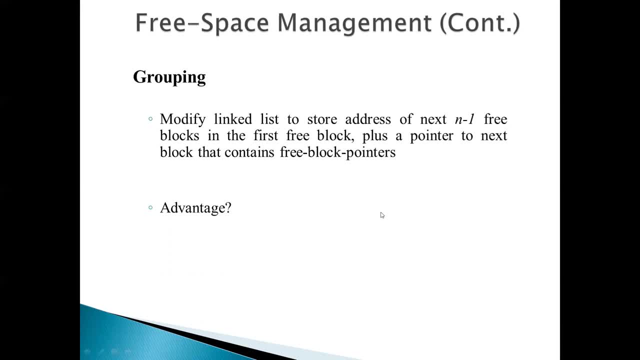 the block is contiguous or not. But here finding address of large number of free blocks is easy. first block is going to contain the addresses of the next n-1 free disk blocks. So finding the addresses of large number of free disk blocks is easy here. 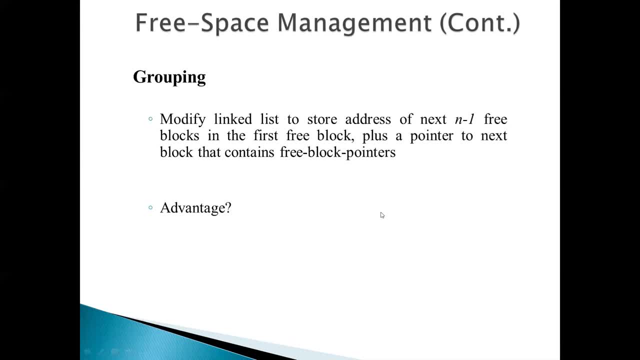 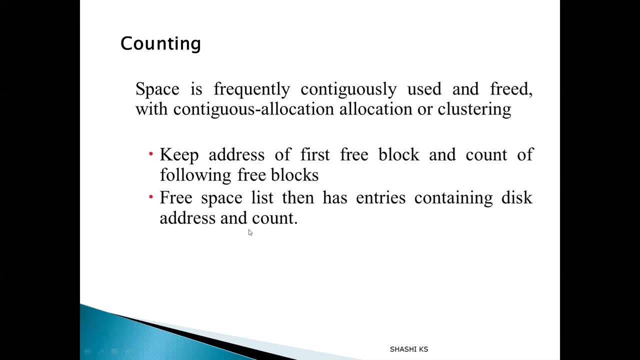 So that is the advantage of the grouping scheme. The last method of implementation of free space management is by using counting, So this is just a modification of our linked list method And this takes advantage of the fact that whenever if you are using contiguous memory allocation algorithm. 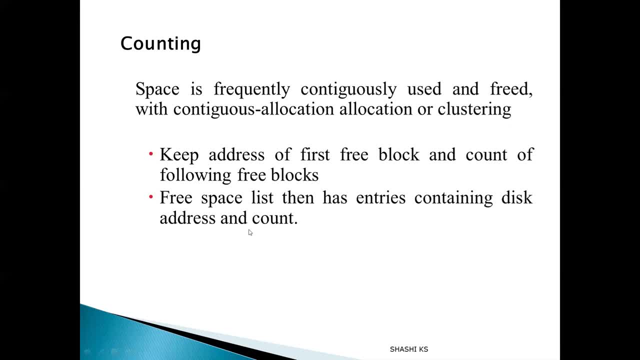 or if you are using some clustering based algorithm, memory is going to be allocated consecutively to a file And when memory is released also, it is going to be released consecutively. Consecutive disk blocks are going to be allocated or released to the file system. 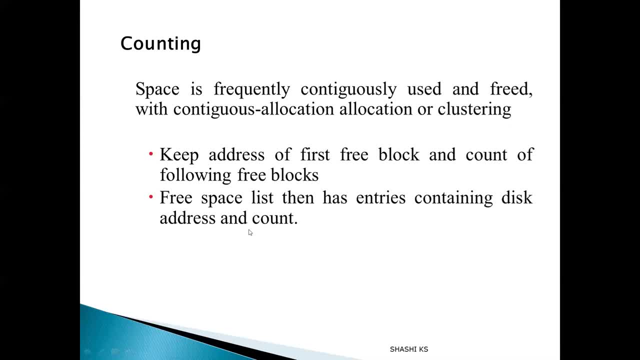 So that means that fact is being taken into account here. So what we do is, in linked list scheme, what we did. so every node, every disk block, will contain the addresses of the next free disk block, right? So here, instead of storing the address of the next free disk blocks, 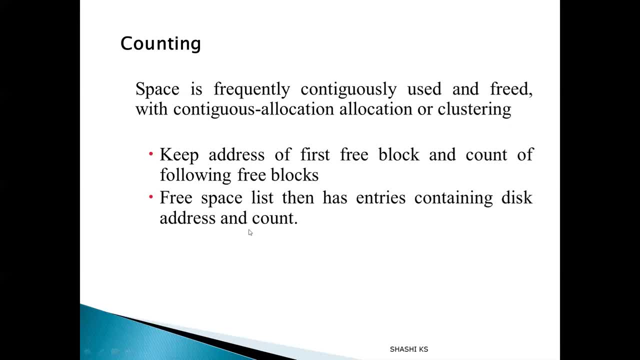 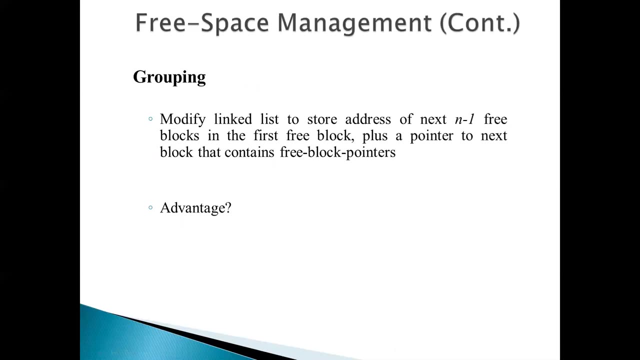 we keep the count of the next free disk blocks. Okay, so the free space header will point to the address of the first free block and the first free block will maintain the count of the following free blocks. Count, not the address. Okay, so in this example, if you take the same example, 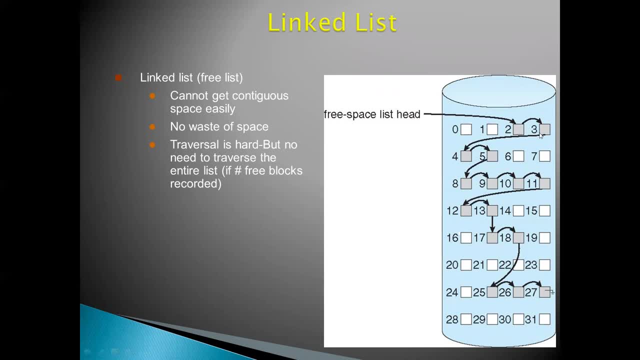 two will contain its own address as well as the count of the following free blocks. How many free blocks following it is free One, two and three. three, four and five are free. That means three, So every first free block, instead of storing the addresses of the next n minus one free blocks. 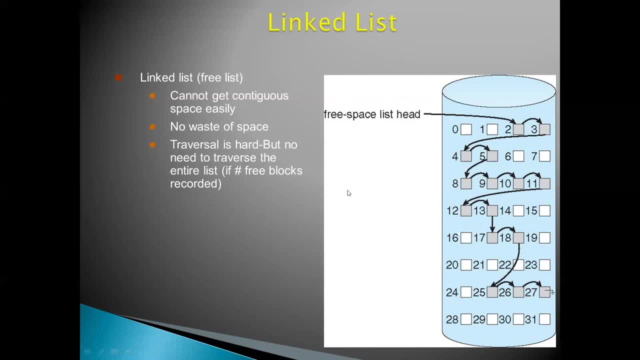 it stores the count of the next n minus one free blocks. Okay, So, so imagine the linked list. So in linked list scheme, in linked list scheme, every node will contain a pointer which points to the address of the next block. 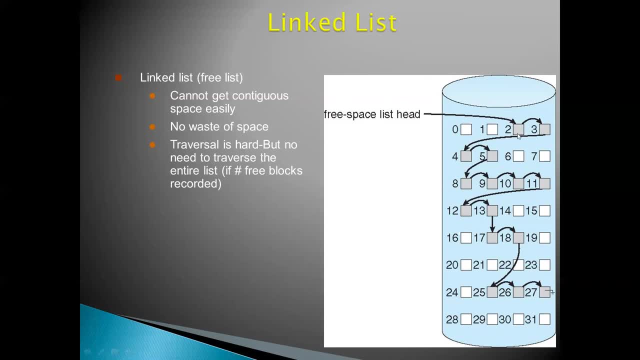 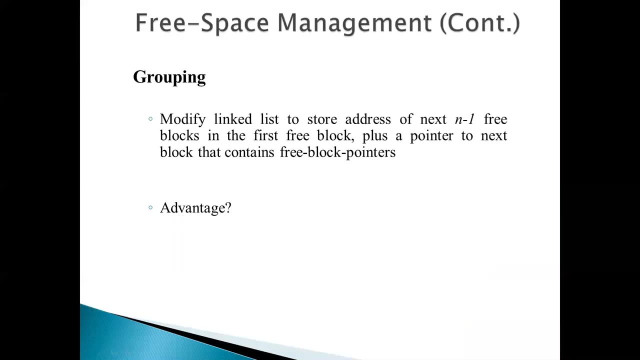 But here it doesn't point to the address, it doesn't store the address, it stores the count of the next n minus one free disk blocks. So that scheme is called as counting. So here each entry in the free space list. free space list. 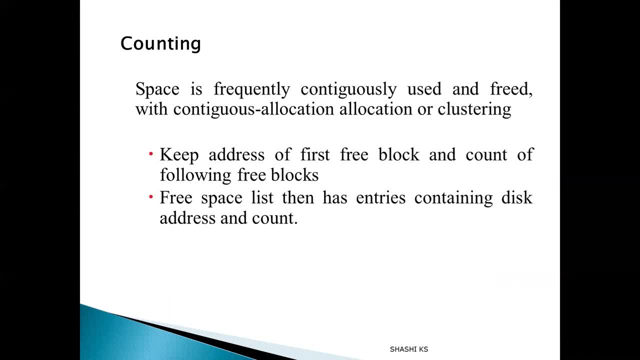 imagine the free space list. it contains an entry of all the free disk blocks, right? So every entry in the free space list will contain the disk, the address of the disk block, as well as a count which tells you how many n minus one free disk. 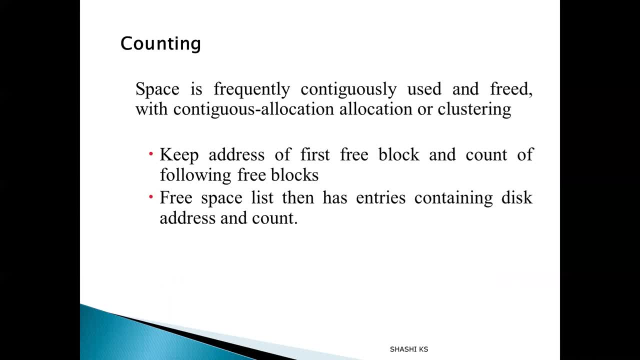 how many disk blocks which comes next to it is free. It contains a count of the number of disk blocks which are free, which are following it, So that scheme is called as the counting based scheme. So when your entry contains only addresses, it is actually. 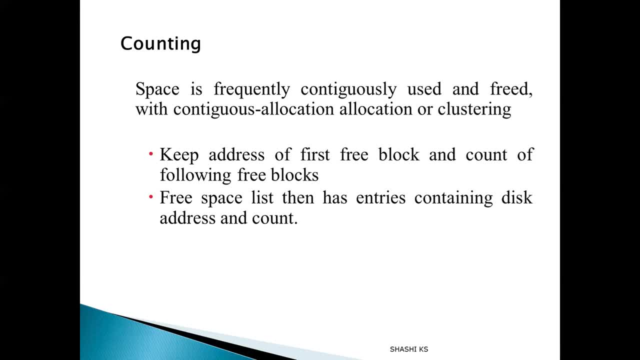 it is actually going to take less space than keeping track of count as well as the address. But then if you have more number of free disk blocks consecutively free, then your number of disk blocks which is going to store the count is going to get reduced. 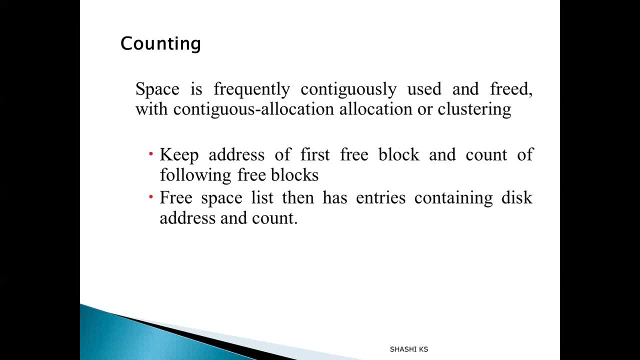 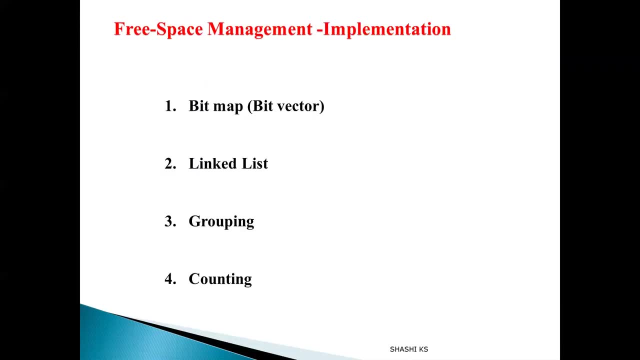 So in that way it is advantageous. So that is all about the different types of free space management implementation. So there are- to summarize, there are- four types of methods of free space management implementation. Free space management generally deals with how to reuse the space on the disk. 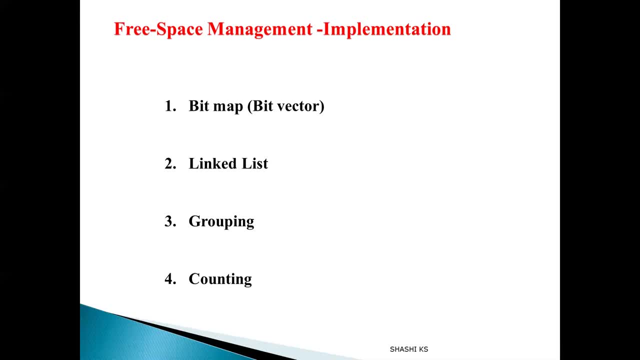 which we get by deleting the files from the disk, And we saw that there are four types of implementation: Implementation by using bitmap, implementation by using linked list, implementation by using grouping and implementation by using counting. So that is all about file system implementation and about free space management.